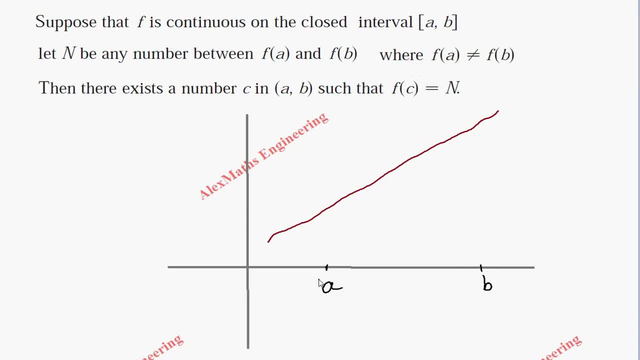 And this function is continuous in this closure interval. a and b, And this value corresponds to the value x, equal to a, is f of a. So this is f of a. In the same way, the value x is equal to b And here, correspondingly, we have f of a. 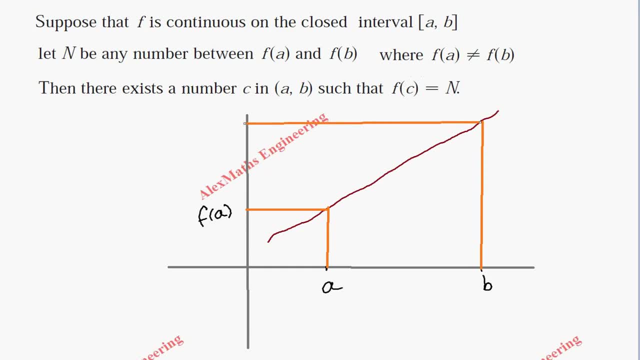 And here correspondingly we have f of b, So we take f of b here. Suppose if there is a number called N between f of a and f of b, So randomly I choose some value capital N here. 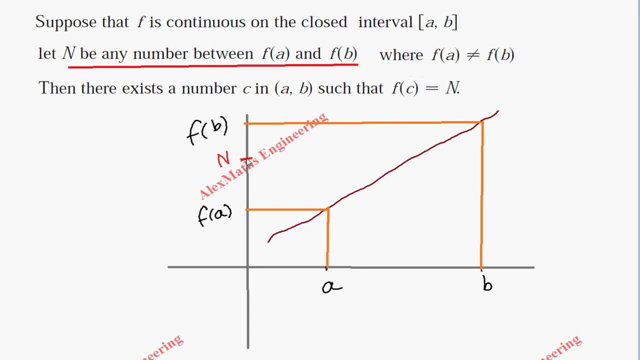 It means this N will have Corresponding x-value called c, which is between a and b. So this f of c will give this N, So this c in a, b open interval, such that f of c equal to N. 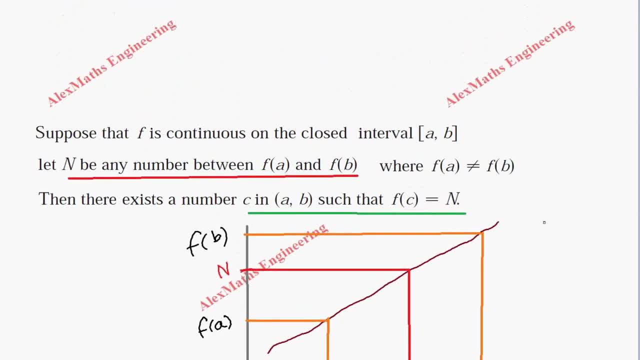 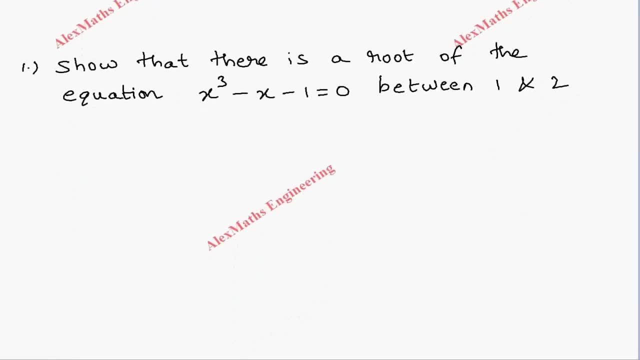 This is what called intermediate value theorem. Using this intermediate value theorem, let's solve few problems. Question number 1.. Show that there is a root of the equation x-x-1 equal to 0 between 1 and 2.. So I will take this as f of x. 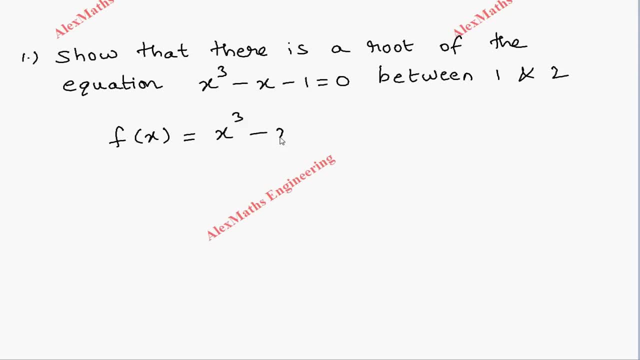 f of x is x-x-1.. Since f of x is a polynomial, it is continuous. Now let's find What is f of 1? f of 1 will be 1 cube minus 1 minus 1.. Totally 1 minus 2, which is minus 1.. 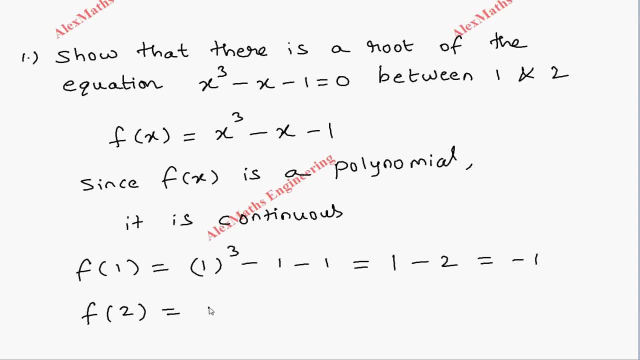 Now let's find f of 2.. So this will be 2 cube minus 2 minus 1.. So this is 8 minus 3, which is 5.. This one is less than 0.. And this is greater than 0.. 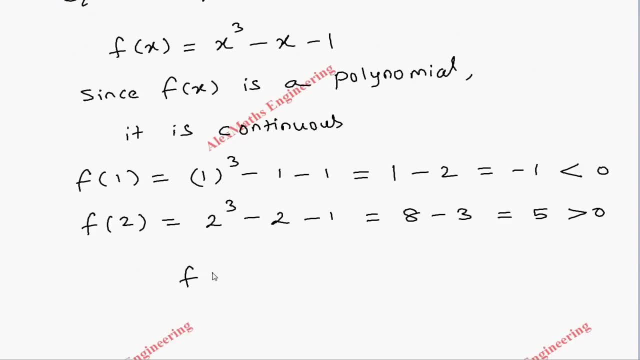 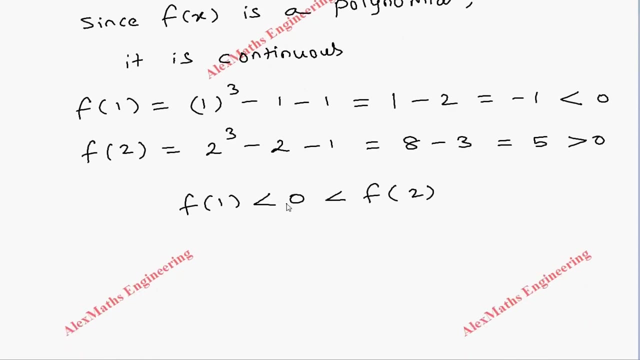 So we can see from these two f of 1 less than 0, which is less than f of 2.. Therefore, it is clear that there is some number c between 1 and 2, such that f of c equal to 0.. 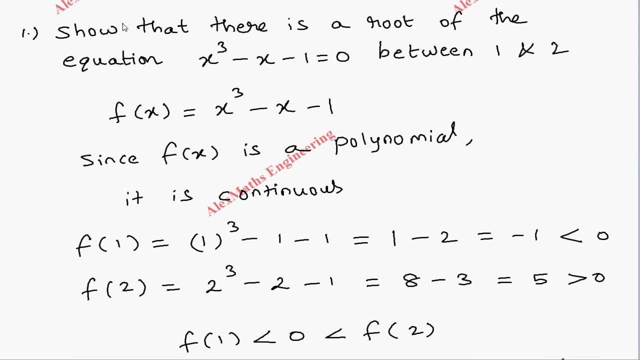 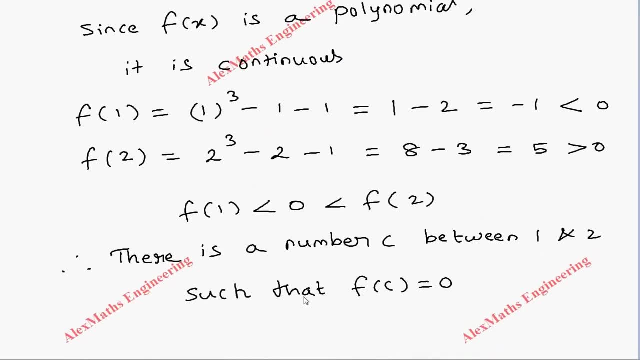 So let's see. So let's see. As for the question, we are asking to show that there is a root between 1 and 2.. Since there is a number c between 1 and 2, such that f of c equal to 0, it confirms that there is a root between 1 and 2.. 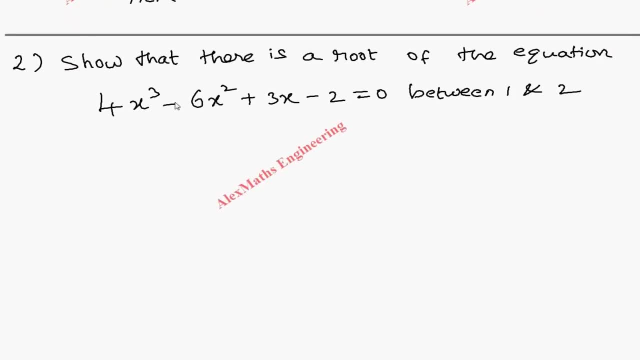 One more similar question Show that there is a root of the equation: 4x cube minus 6x square plus 3x minus 2, equal to 0, lies between 1 and 2.. So let's name this polynomial as f of x. 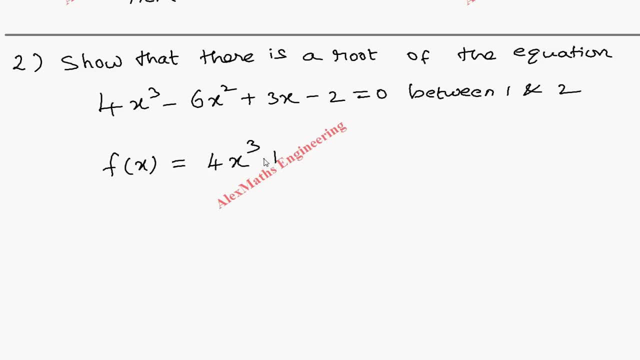 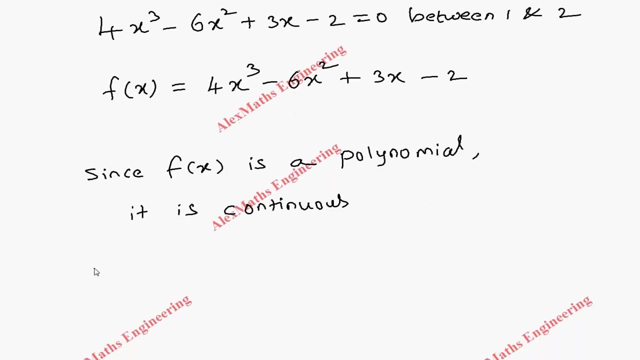 So it is 4x cube minus 6x square, plus 3x minus 2.. Since it is a polynomial, it is continuous. We can state like a previous sum, And after that we are going to find what is f of 1.. 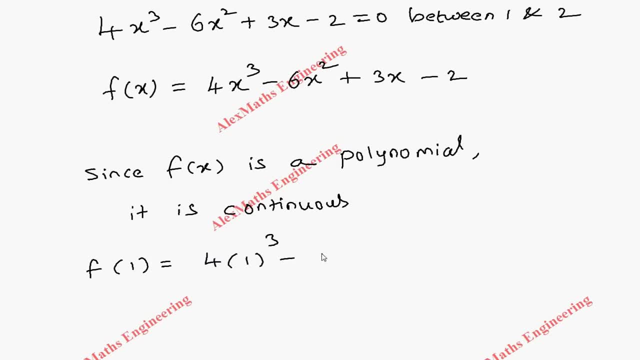 So 4 into 1 cube minus 6 into 1 square, plus 3 into 1 minus 2.. Which is 4 minus 6 plus 3 minus 2.. Totally minus 1, which is less than 0.. 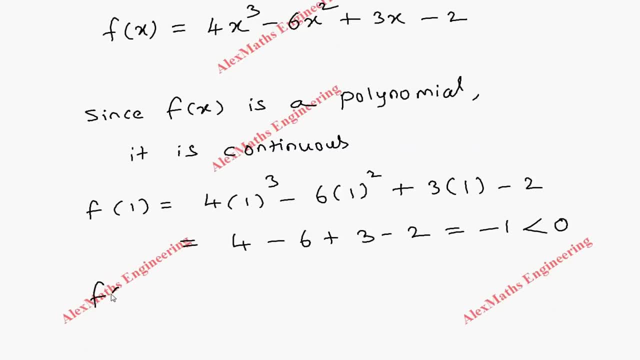 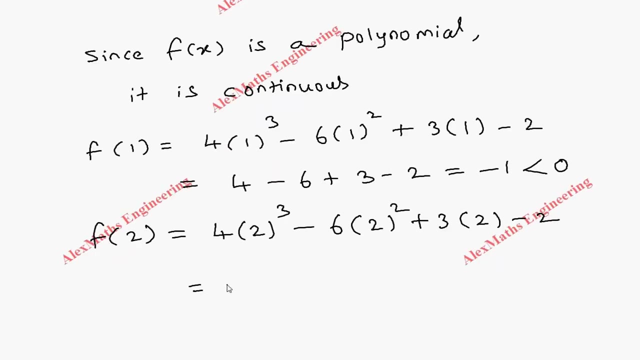 And now let's calculate f of 2. Which is 4 into 2 cube minus 6 into 2 square plus 3 into 2 minus 2.. This will give 4 into 2.. 8 minus 6 into 4 plus 6 minus 2.. 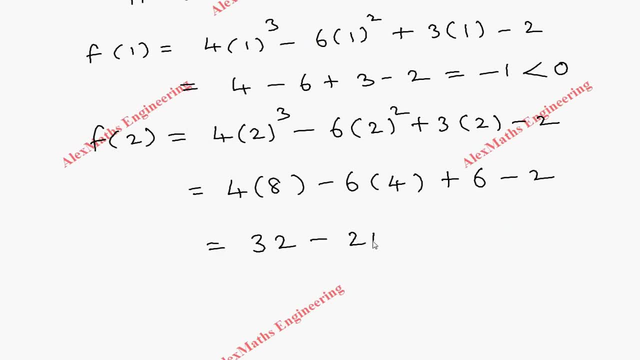 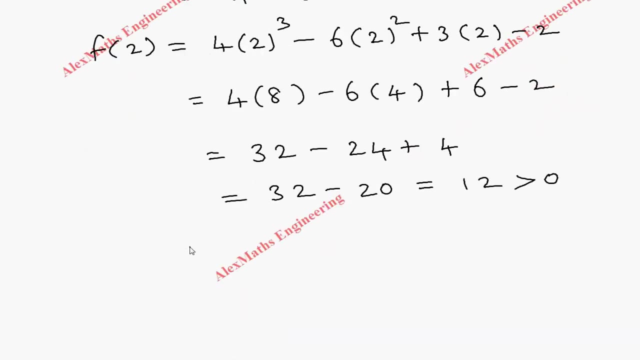 This is 32 minus 24.. And these two after simplification, plus 4.. So this is 32 minus 20, which gives 12. Which is more than 0.. So from this we can see f of 1 is less than 0..